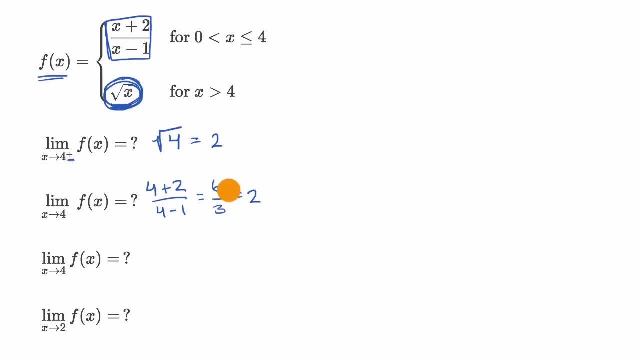 to have a limit, you have to be approaching the same thing from the right and the left, And we are, and so this is going to be equal to two. Now, what's the limit? as x approaches two of f of x? Well, as x approaches two, we are going to be completely. 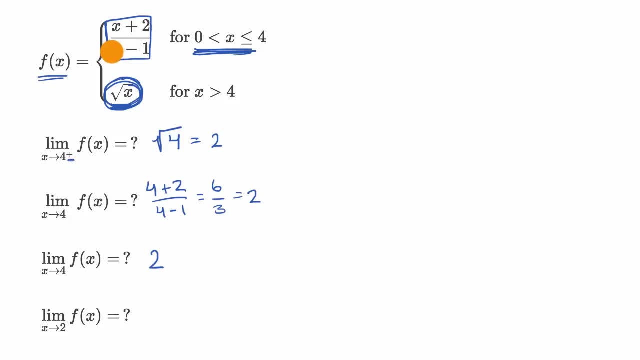 in this scenario right over here Now, interesting things do happen. at x equals one- here Our denominator goes to zero. But at x equals two. this part of the curve is continuous, so we can just substitute the value. It's going to be two plus two over two minus one. 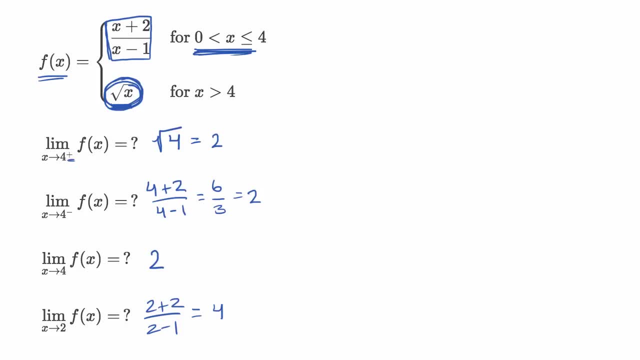 which is four, over one, which is equal to four. Let's do another example. So we have another piecewise function, And so let's pause our video and figure out these things. All right, now, let's do this together. So what's the limit as x approaches negative one? 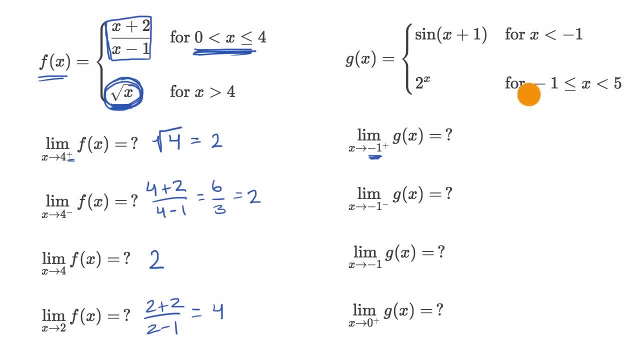 from the right. So if we're approaching from the right when we are greater than or equal to negative one, we are in this part of our piecewise function And so we would say this is going to approach, this is going to be two to the negative one power. 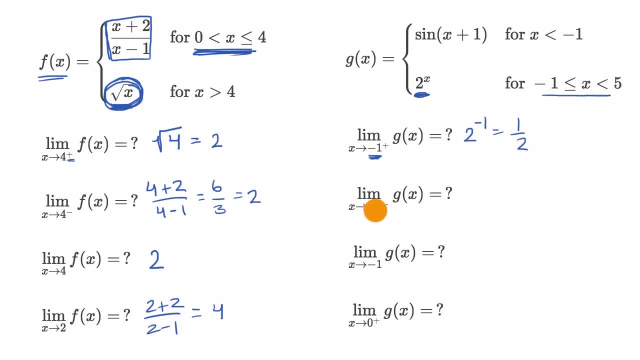 which is equal to 1 1⁄2.. What about if we're approaching from the left? Well, if we're approaching from the left, we're, in this scenario, right over here. We're to the left of x equals negative one. 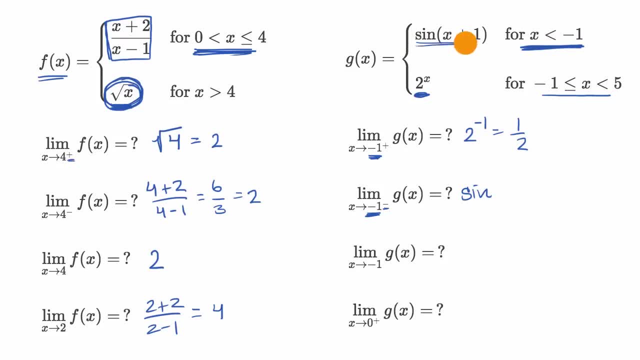 And so this is going to be equal to the sine, because we're, in this case, for our piecewise function of negative, one plus one, which is the sine of zero, which is equal to zero. Now, what's the two-sided limit as x approaches negative? one of g of x. 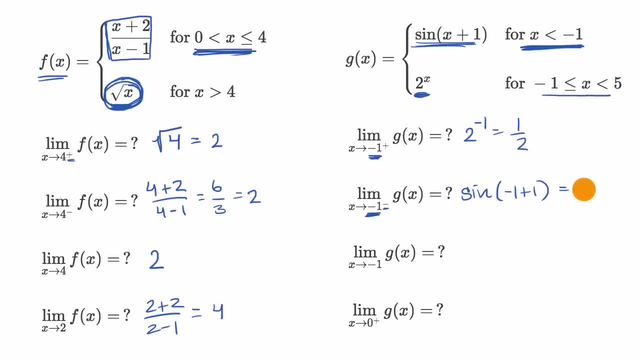 Well, we're approaching two different values, as we approach from the right and as we approach from the left, And if our one-sided limits aren't approaching the same value, well then this limit does not exist, Does not exist. And what's the limit of g, of x? 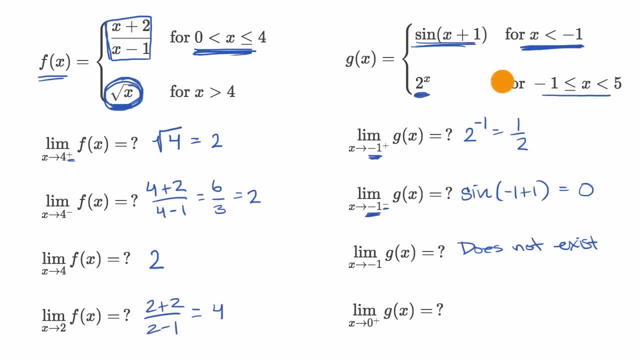 as x approaches zero from the right. Well, if we're talking about approaching zero from the right, we are going to be, in this case, right over here. Zero is definitely in this interval And over this interval, this right over here, is going to be continuous.